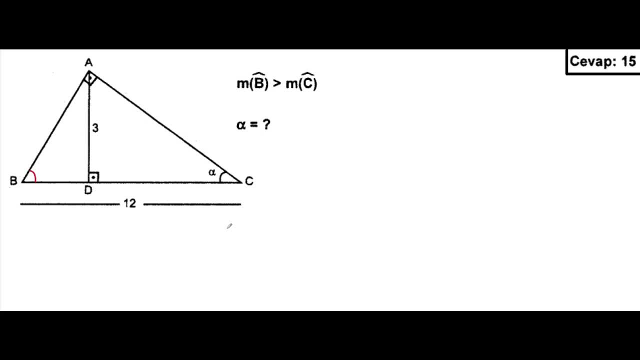 Hi everyone, welcome to the channel Universal Math. In this video, I'll try to explain the solution of this problem. Before starting, don't forget to subscribe to my channel and press the like button. So let's get started. We're given that the angle B is greater than the angle C. 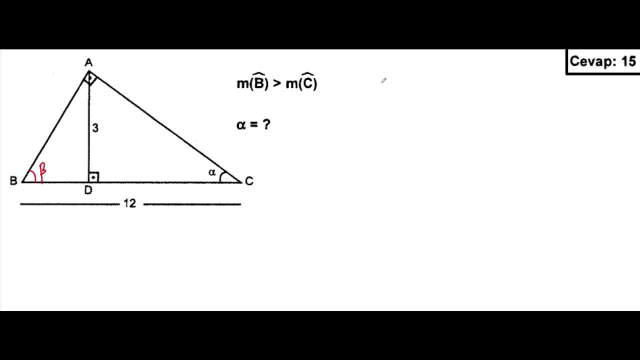 So we can write down this angle as beta and beta is greater than alpha. We'll write it down, Okay, here, alpha, And we know that this angle is 90 degrees, which means that beta is greater than 45 degrees. 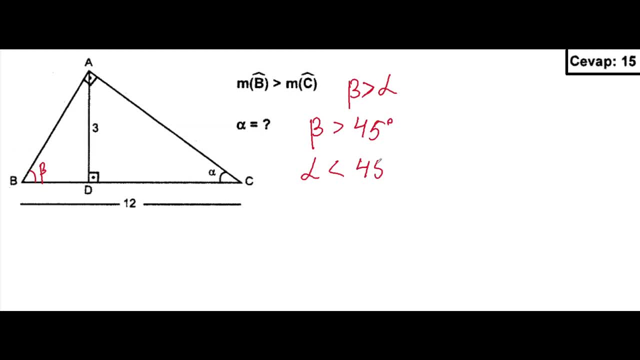 and alpha is less than 45 degrees. It will help at the end And we'll write down the answer So we can use here sine's theorem And here sine alpha. Sine alpha will equal to here 3 over. we can write down a C side as any letter like B. 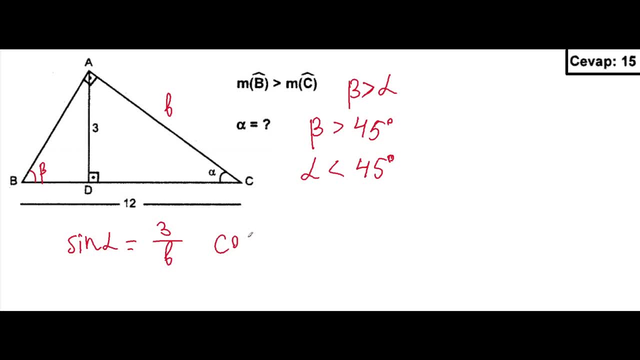 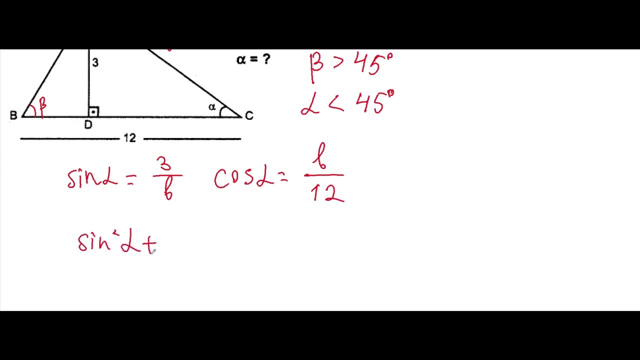 And write down B, 3 over B and cosine alpha here will be equal to. in a big triangle it will be B over 12.. And we know the formula: Sine squared alpha plus cosine squared alpha is equal to 1.. 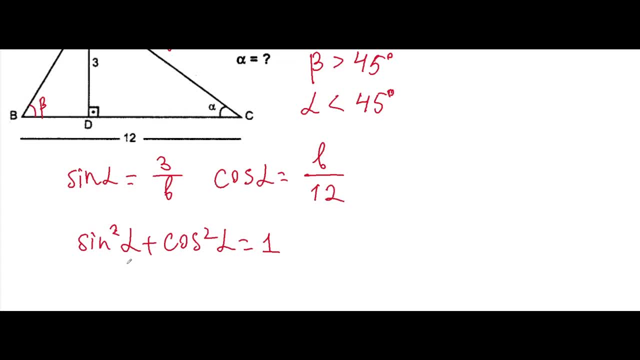 And we can plug it here. Plug these two expressions here and we'll get 9 over B squared, plus B squared over 144.. 144 will be 8.. It'll be equal to 1. And we can multiply it by B squared times 144.. 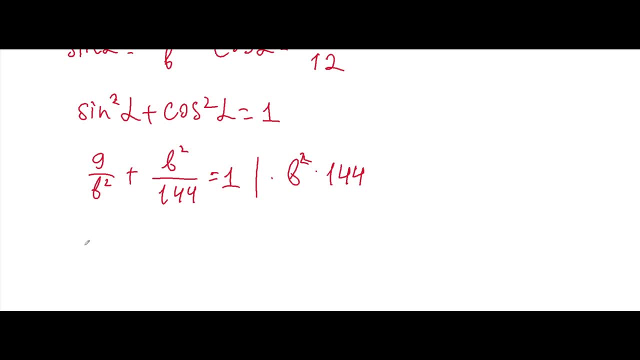 And we will get here. the first will be 9 times 144, plus B fourth degree and two equal to B squared times 144.. Okay, Let's try it from the both sides. size this expression and we'll get here b fourth degree minus b, 144 times times b squared. 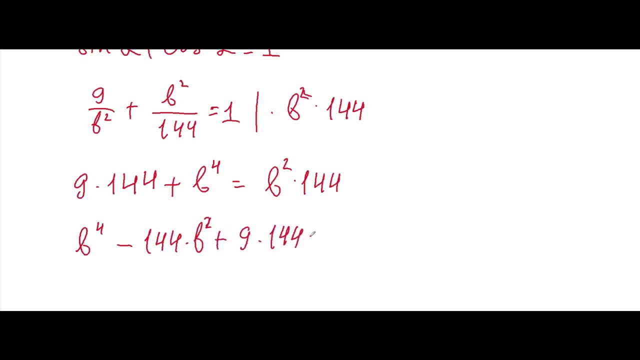 plus 9 times 144 will be equal to 0.. we can use here uh discriminate will be equal to 144 squared minus 36 times 144, and it seems at the first shot very difficult, but it's not difficult, believe me here. 144 squared minus here's 36 is a square. 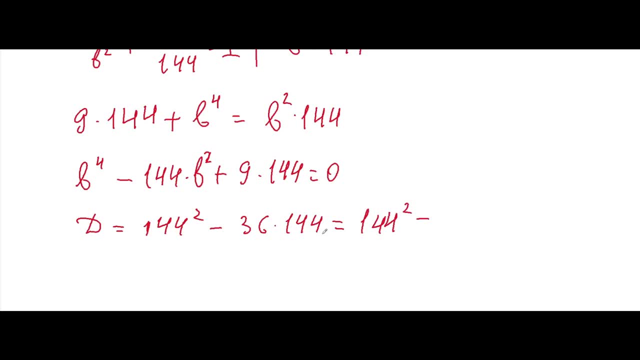 square of 6, and 144 is a square of 12.. so 12 times 6 will give us 72 and this is all squared. here it was like this: all is squared and we got this and we can write down this as 144 minus 72 times 144 plus 72. 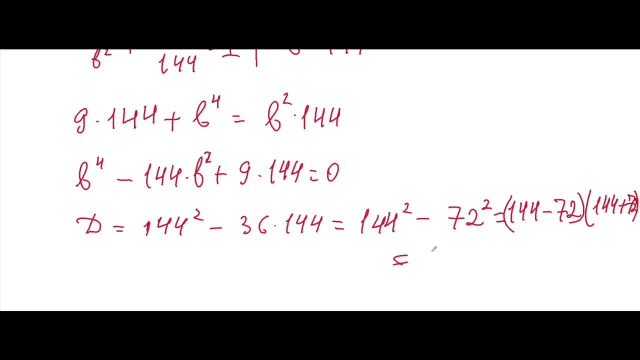 and it will equal to here 72 times. here it will be 216 and this will equal to here. 216 is a 6 cube and 72 is 6 times 12 and we can write down it as 6 fourth degree times 12 and 12. we can also write down as: 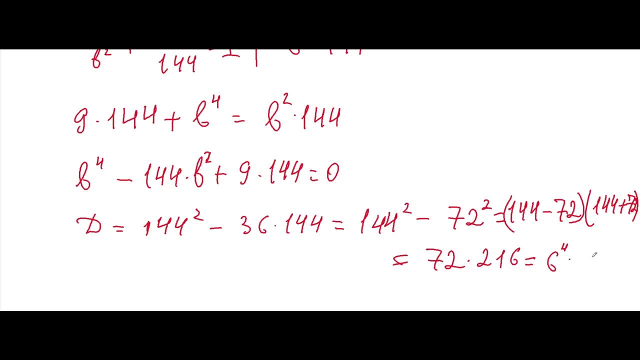 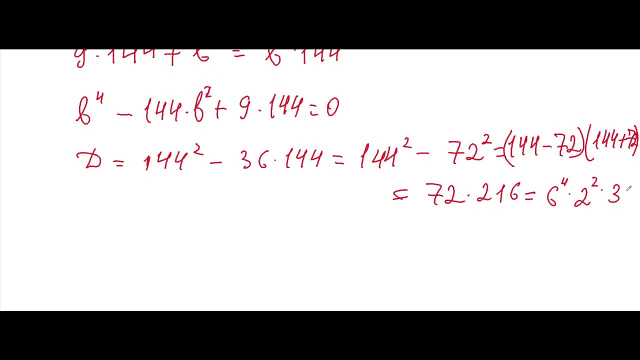 72.. four times three, it is two squared times three. and here we can write down this, all this as 31 squared and 31 squared times 2 squared, we can write down this as 72 squared, 72 wrong and 3. we can write down square root of 3 squared. this will be square root of 3. 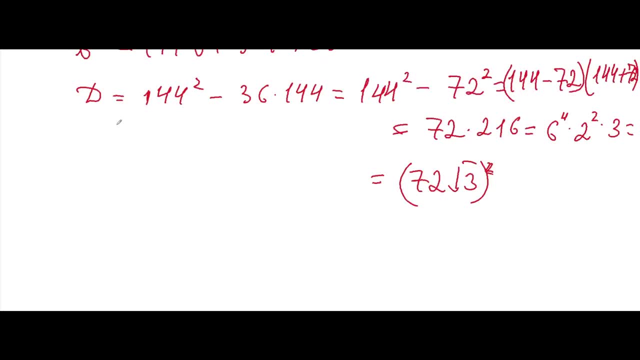 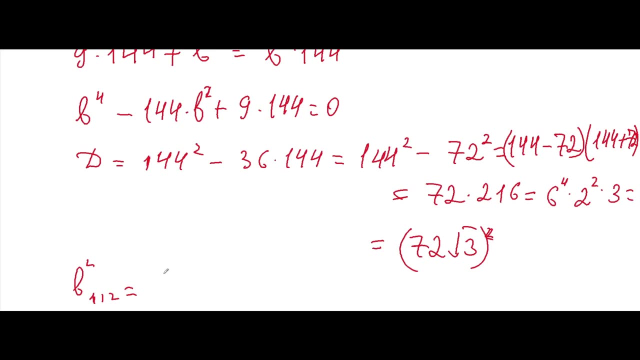 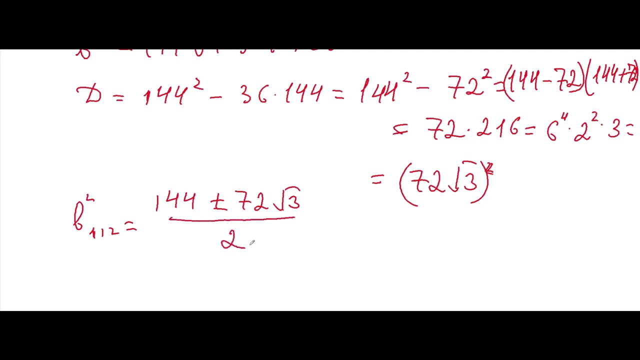 all this squared and we can write down that B squared 1, 2 will be the first and second will be 144 plus minus 72, square root of 3. we write down it- and over 2. see here, it is accurate here and it will equal to 72 plus minus. 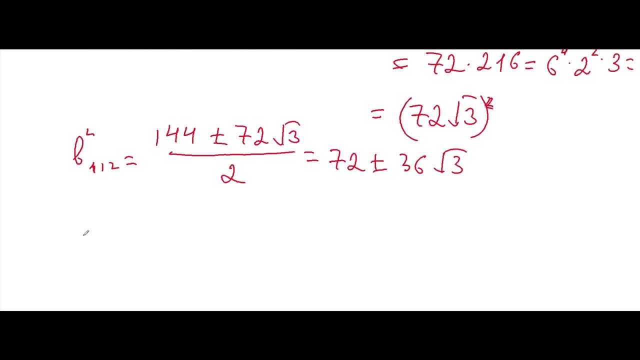 36 squared of 3, and I can write down B squared of 36 times 2 plus minus squared of 3, and here it will equal to 3 squared over 74. so that is measured throughout a warehouse times two plus minus square root of three. 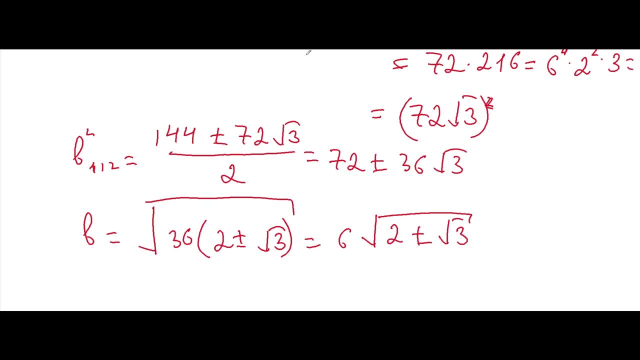 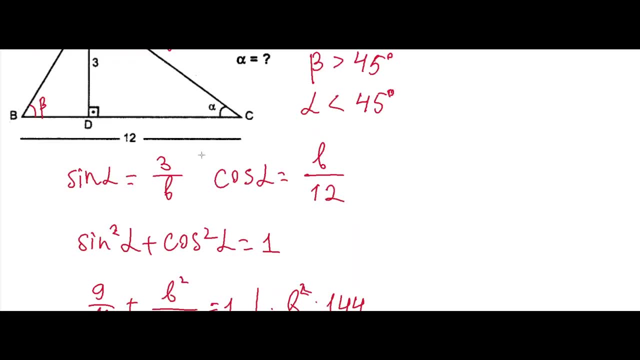 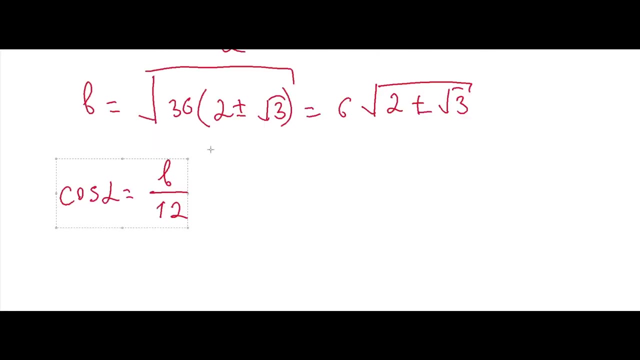 it will not be plus minus because this side cannot be negative number. so we can plug instead of b here let me copy this: so now we can plug this instead of b here and we'll get here that cosine alpha is equal to six times square root of two plus minus square root of three. 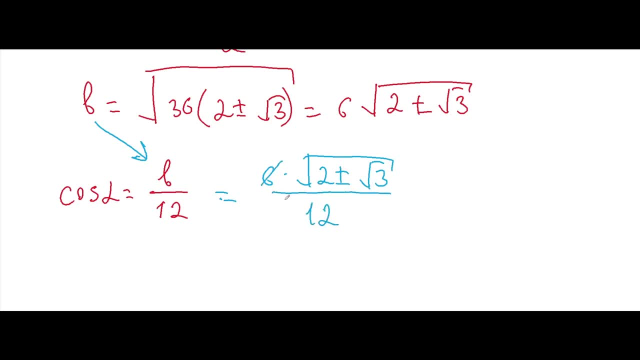 over twelve and we can cancel it and we can get here, uh, square root of two plus minus, square root of three over four, it will be all this in a square root. i believe you understood this, and cosine alpha here have to be um, square root of one plus minus, square root of three over two. we can write down over two. 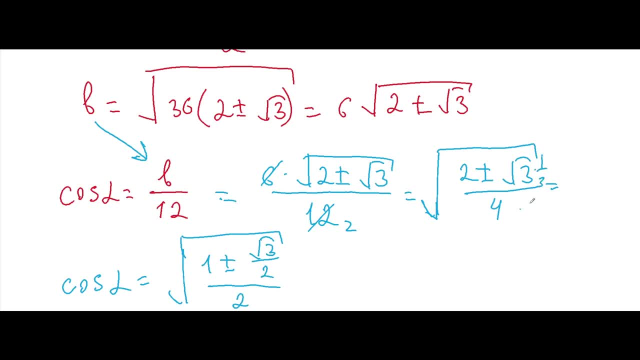 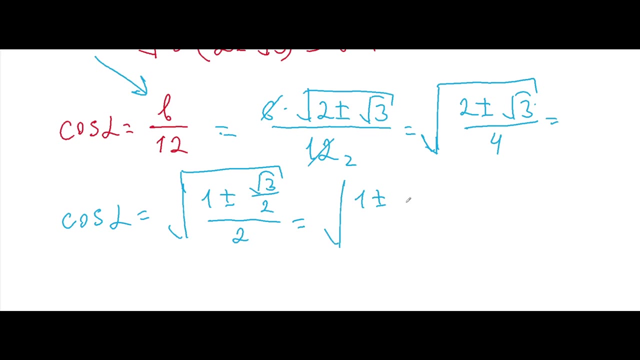 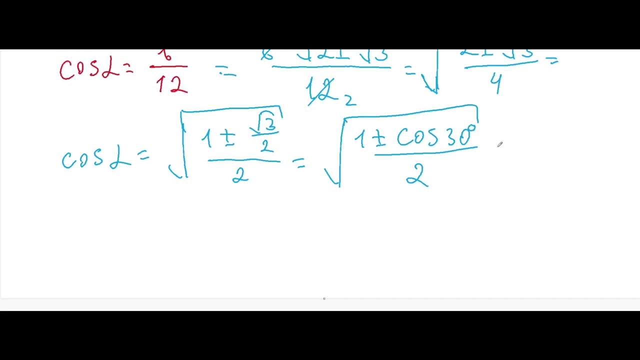 i multiplied the both numerator and denominator by one over two, divided by one over two, and got this expression: and we know that square root of three over two is here: cosine 30 degrees plus minus, cosine 30 degrees over 2, and we know that this expression is equal to: 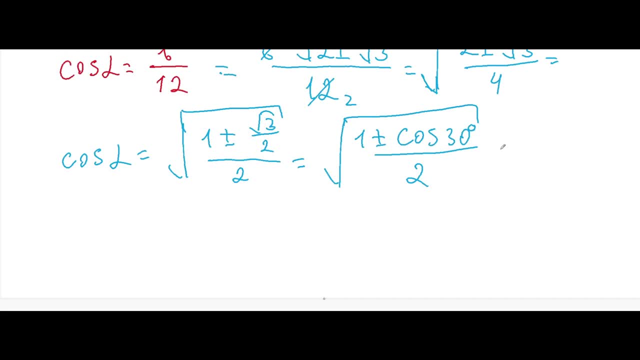 15 degrees or cosine. yeah, it is equal to cosine 15 degrees or cosine 75 degrees. why is it so? I will just write down it to prove this. Cosine 30 degrees. we can write down this as in a two ways: cosine alpha will be equal to the first one and